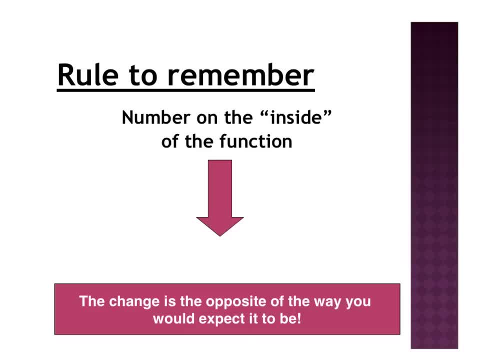 It's on the inside, and that's when you have a horizontal transformation. Otherwise it would be vertical. We also need to remember that the change is the opposite of what you'd expect. So if I'm adding 7 inside the function, you're actually moving to the left 7.. 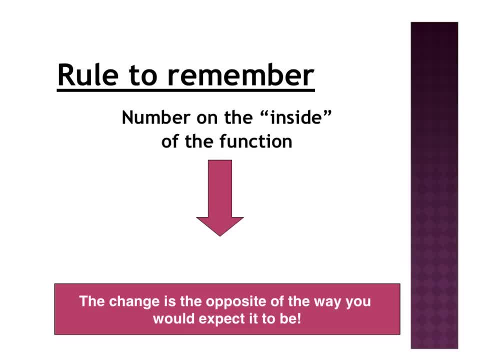 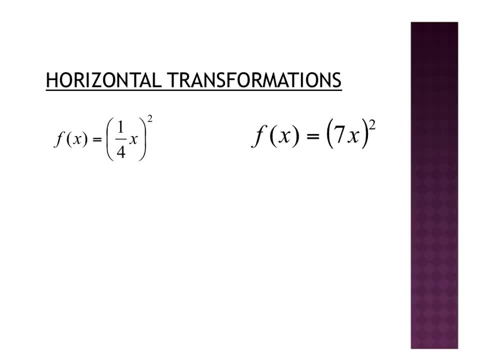 If I'm multiplying by 1 fourth, on the inside of the function I have a vertical stretch by a factor of 4, because I flipped that, So you've got to think opposite when we're doing horizontal. Let's try a couple examples here. Here I have: the f of x equals 1 fourth x. 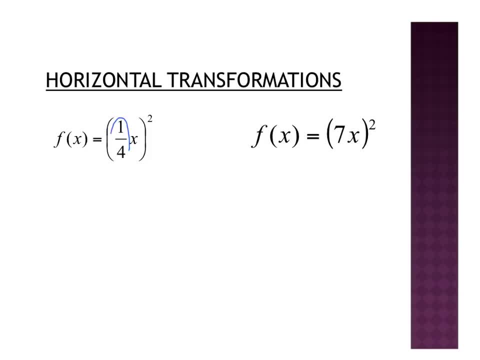 And all of that is squared so that 1 fourth inside the part that's being squared causes it to be a horizontal transformation. Now I have to think opposite. so my factor is going to be 4, because I'm going to flip that 1 fourth, so I'm going to have a horizontal stretch by a factor of 4.. 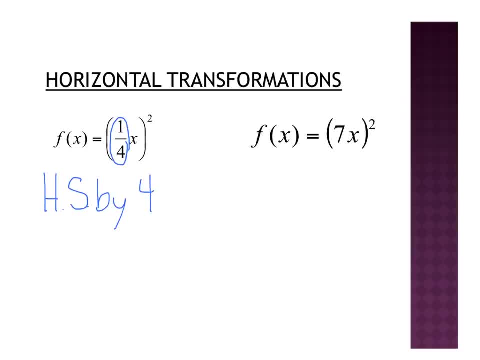 I like to think of my factor before I write down horizontal stretch or compression. Now, here I have a 7.. Well, okay, I know it's going to be horizontal because it's on the inside, That's good, And my factor is going to be actually 1. seventh, because I have to flip it. so I'm going to have a horizontal compression. 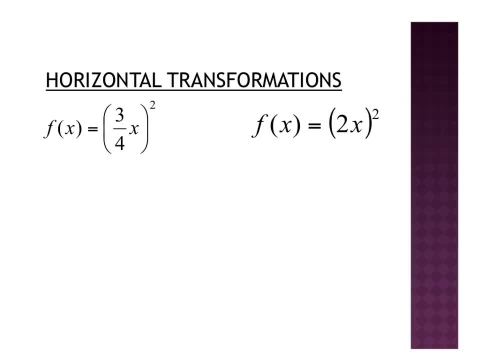 I want 7.. Let's try a couple more. Here. I have 3 fourths x and all that's squared. Well, I know it's going to be horizontal because it's on the inside. Now, when I flip that, I have 4 over 3.. 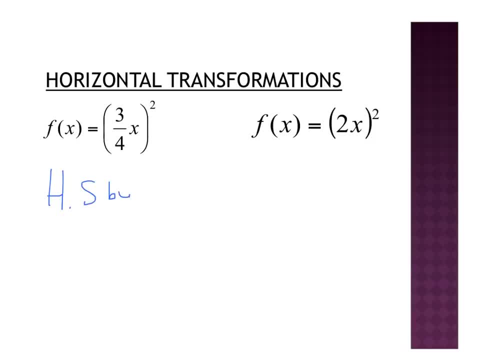 Well, 4 over 3 is greater than 1, so it's going to be a horizontal stretch by 4 thirds. And lastly, on this one we have a 2.. Well, I know it's going to be horizontal because it's being squared, It's on the inside of the function. 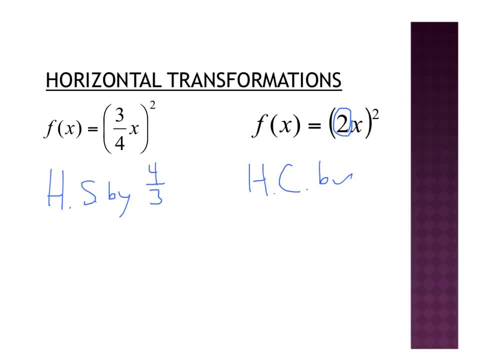 And I'm going to have a horizontal compression by 1 half. Remember, our factor is going to be 1 half. because I have to think opposite. I have to flip it when it's inside the parentheses. Last two will be a couple combos here. 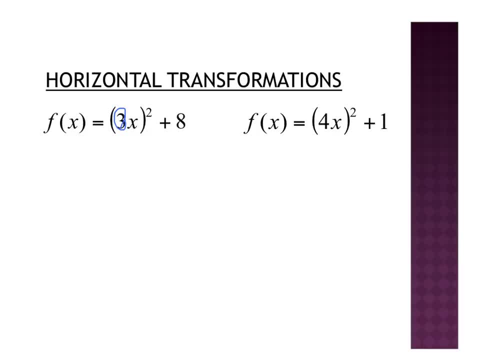 Inside I have this 3.. That 3 is being squared. so I know that's a horizontal transformation of some kind. Well, I have to think okay, well, it's going to be 1 third, because I have to think opposite. 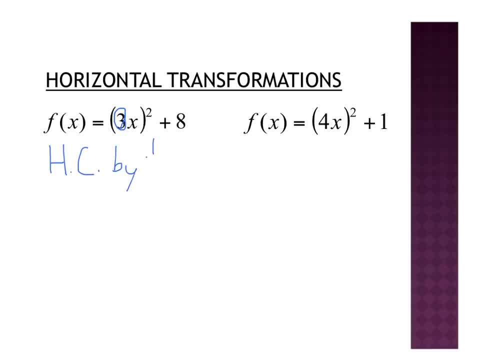 I have to flip it so I have a horizontal compression by 1 third. Here I have an 8. I'm adding 8. Well, it's outside, so it's vertical When I'm adding it's uppercase And, I think, regular. so I'm going to go up by 8..